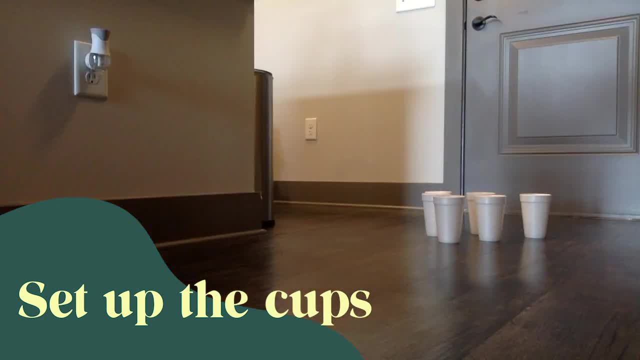 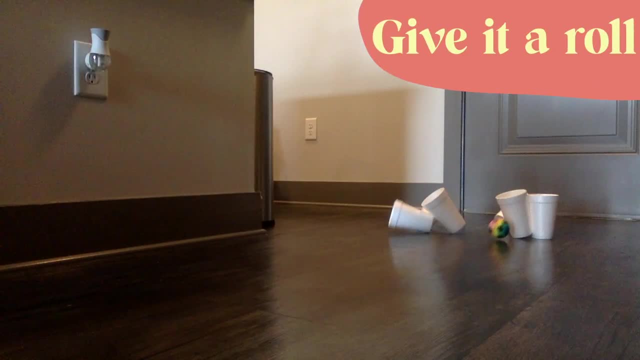 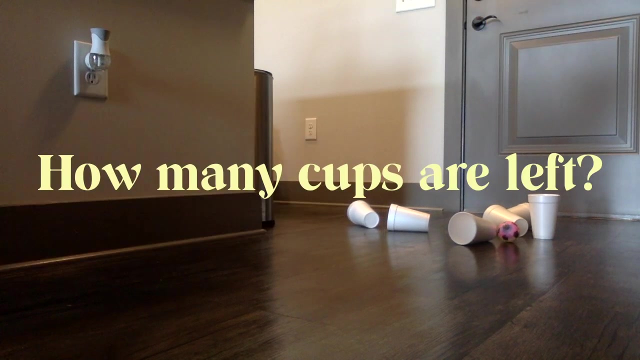 going to set out all of your cups just like you would with bowling pins. Once you are done doing that, then you can take your ball and have at it, Give it a roll. As you can see, I started out with six cups standing. then five fell over How many cups are left. So that means six minus five must. 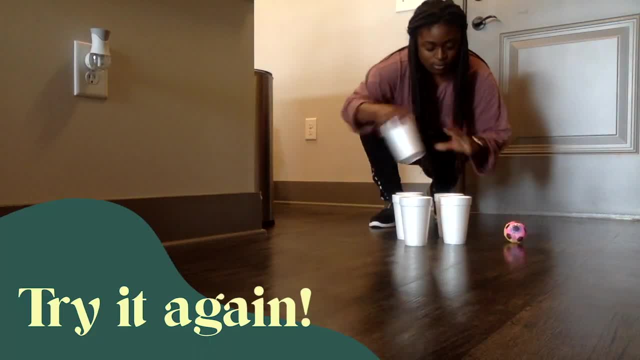 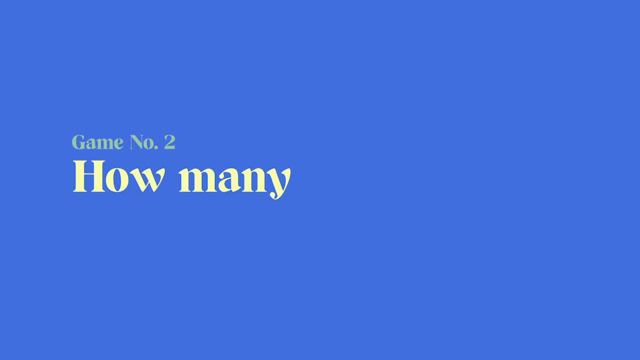 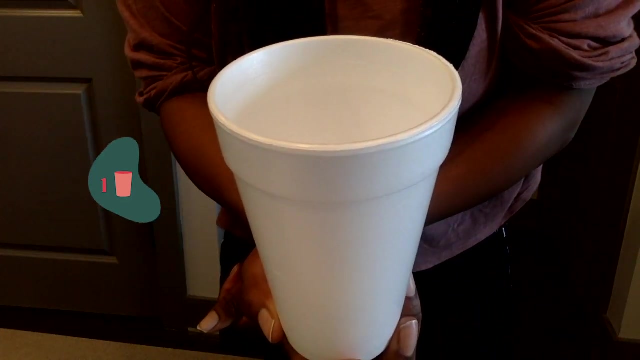 be one. When you're done, you can set it up again and you can try it again with another bowl. This next one is called how many are many? Next, you'll need 10 pennies and a cup. Okay, so let's get started. You're going to take your 10 pennies and you're going to lay them all. 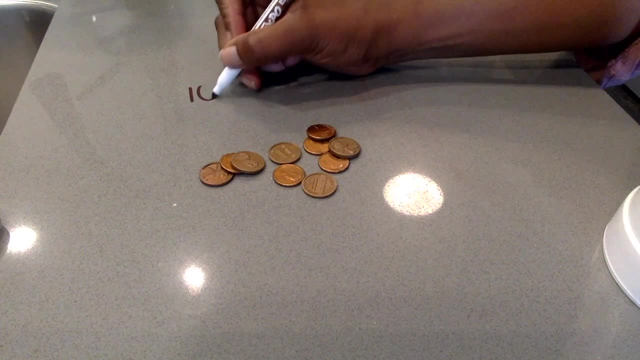 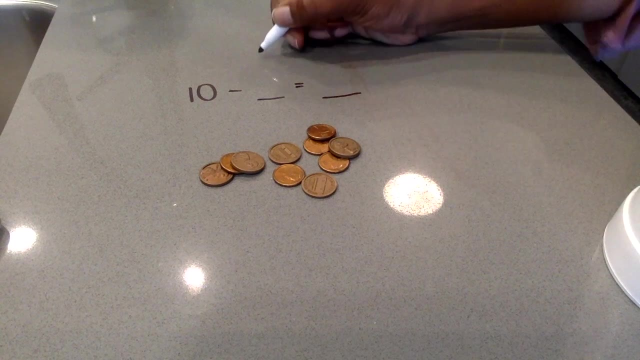 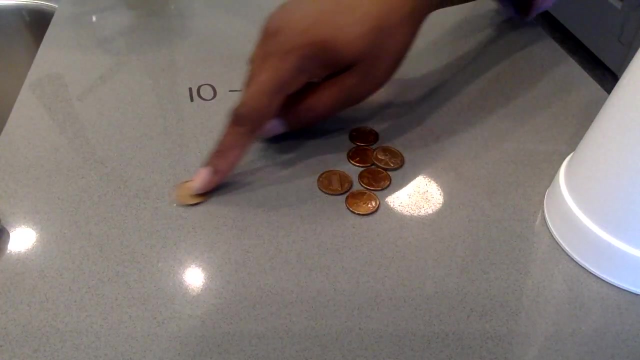 out. Then we're going to write the number 10, because we're starting out with the number 10 and we're going to try to figure out how many are missing in the cup. Next, you're going to close your eyes, use your cup to cover up some of the pennies, then open your eyes. 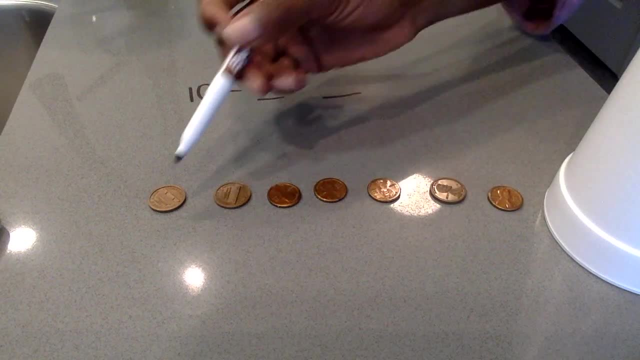 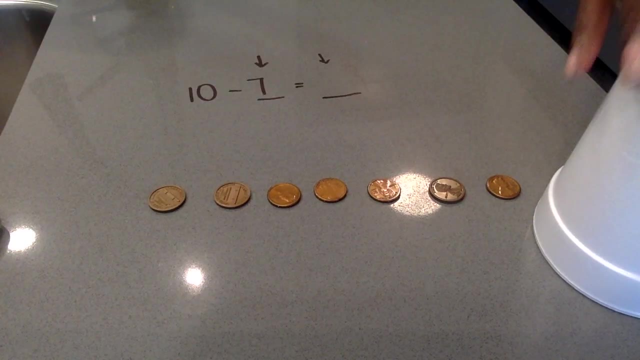 and then you're going to take your 10 pennies and you're going to lay them all out. We're going to count and see how many pennies are left from outside of the cup. Here we are left with seven. Now we need to figure out how many are in the cup. 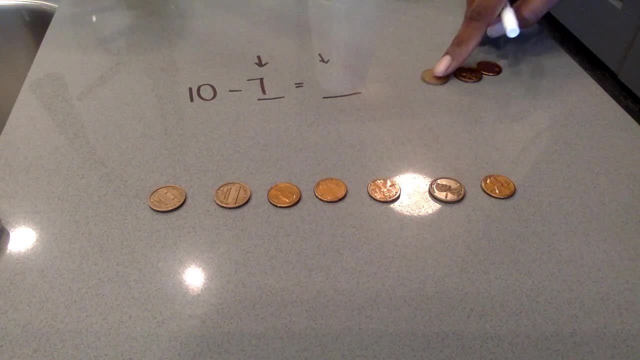 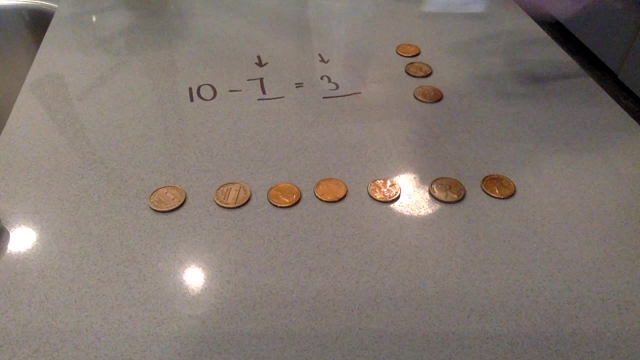 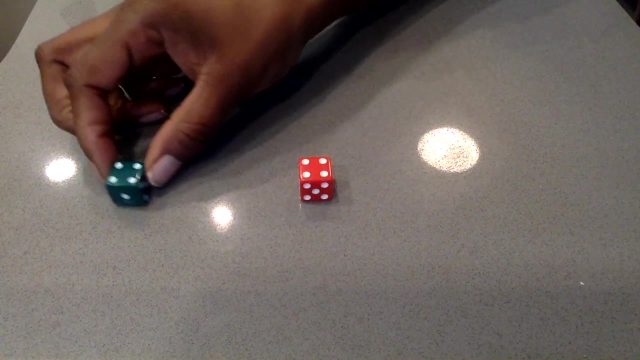 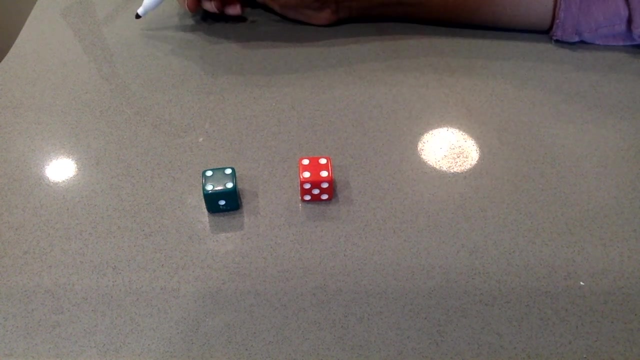 how many are missing? Three, One, two, three. There were three pennies missing from our group. 10 minus 7 equals 3.. Next, we have dice subtraction, which is similar to dice addition, but the only difference between dice subtraction and dice addition is that you want to make sure the bigger 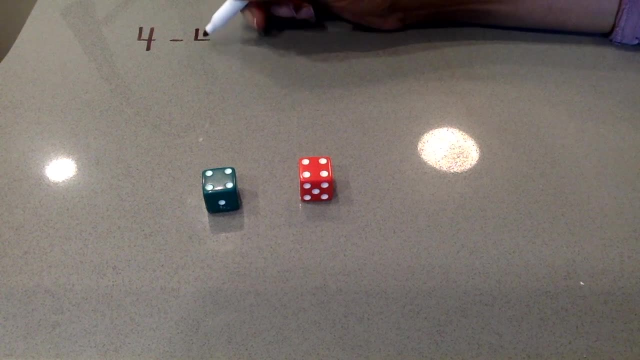 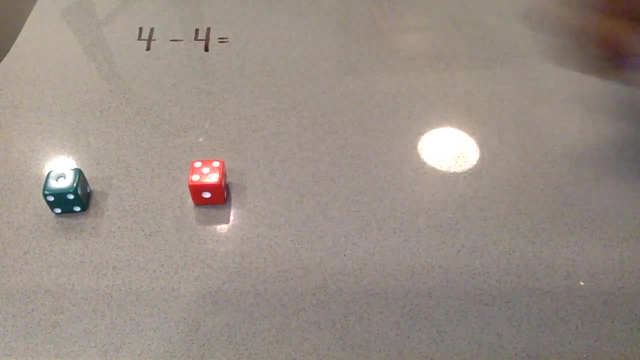 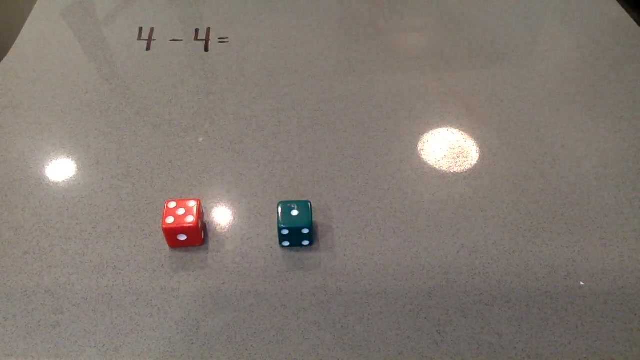 number always goes first, because you cannot take away from a smaller number. Here we have 4 minus 4.. They're both the same number, so it doesn't matter which 4 you decide to write first. Our next one says 5 minus 1.. Five is a number that is bigger than one, so it has to be written first.